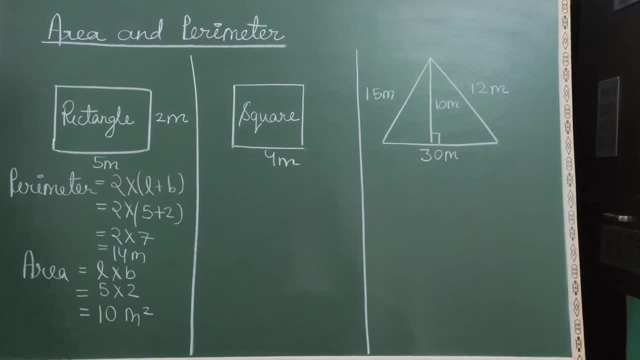 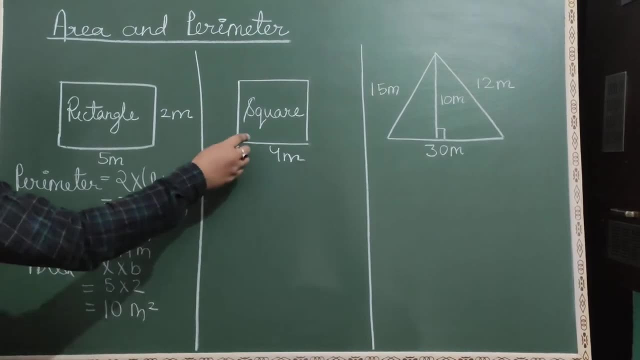 be meter, but this is area, so here will be meter square. So the unit of area of rectangle is meter square. Now here we are finding the perimeter of rectangle. So here we will make a creep according to the number of WILL Here. first we have to find the perimeter, So here we have to find. 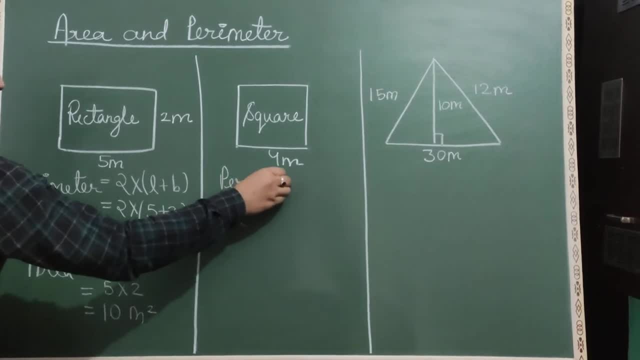 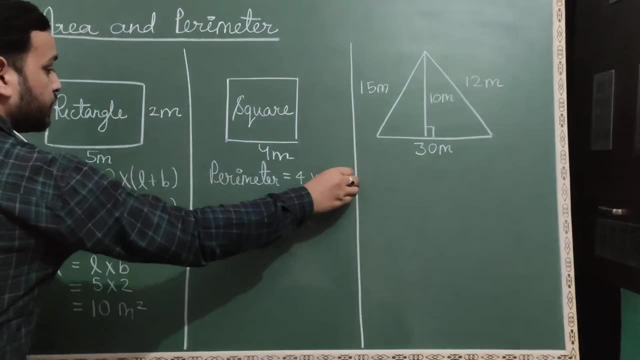 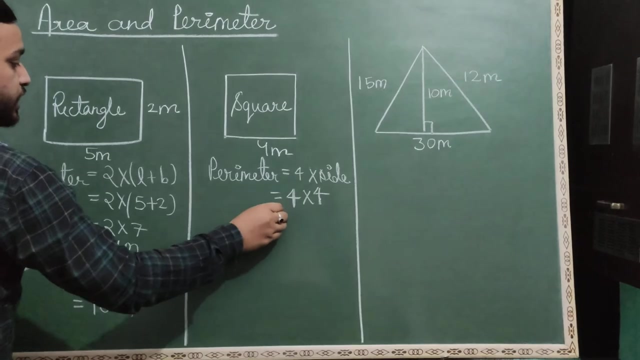 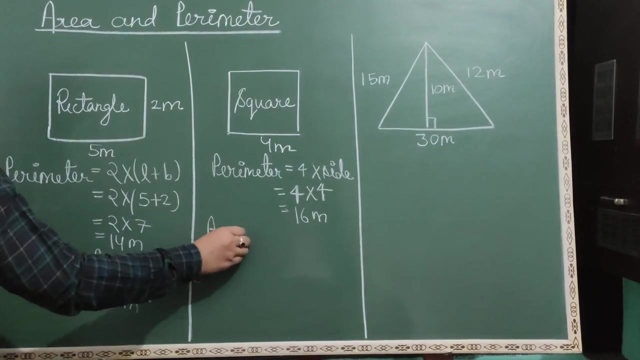 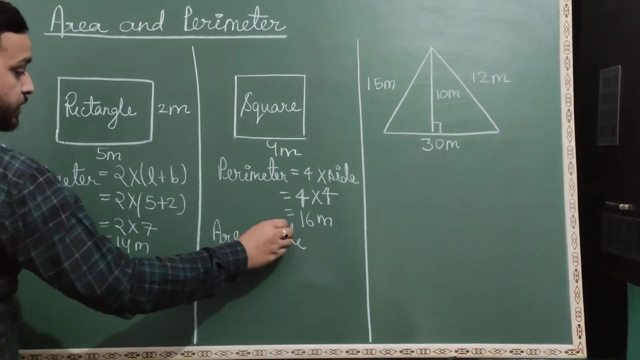 of square. Now, perimeter of square formula is 4 multiply side. Now here you can see side is what is the length of the side. this is 4.. So 4 for the 16 meter Now area of square. area of square will be side into side. So side multiply side, Side multiply side Now. 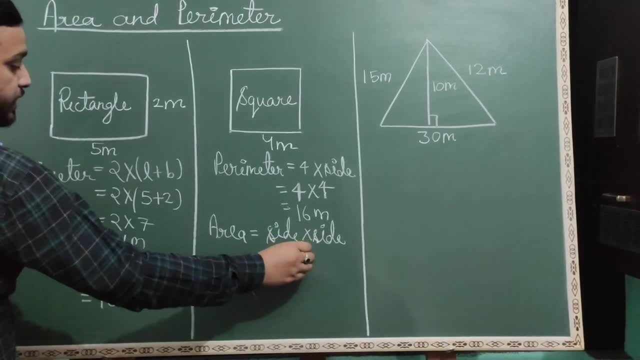 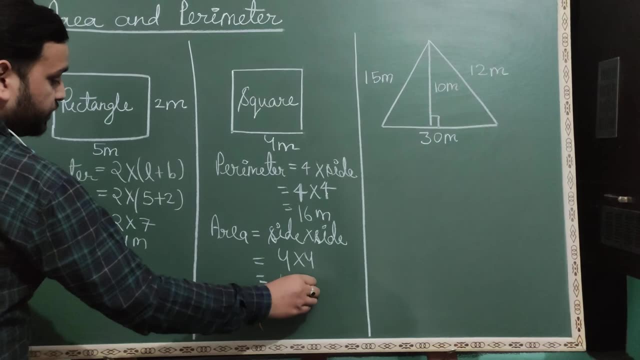 side is 4 and another and same again, 4, because all sides of square are equal. that is why 4 into 4, 4 for the 16. Now the unit will be meter square. It is not meter, it is meter square. 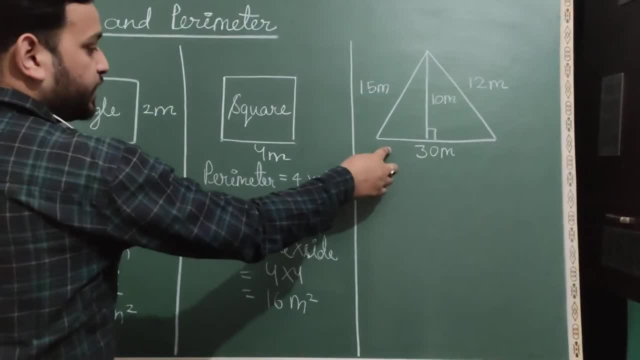 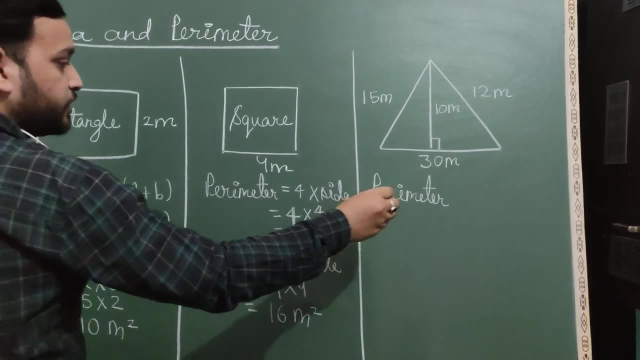 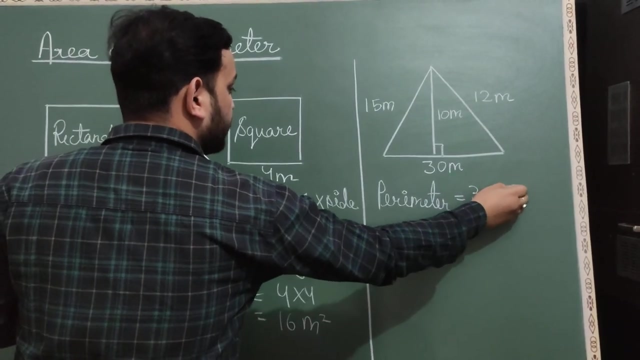 Because this is area. Now, third one: this is triangle. So perimeter of triangle is sum of all 3 sides. So we will add all 3 sides: 30,, 15 and 12.. 30 plus 15 plus 12.. You are. 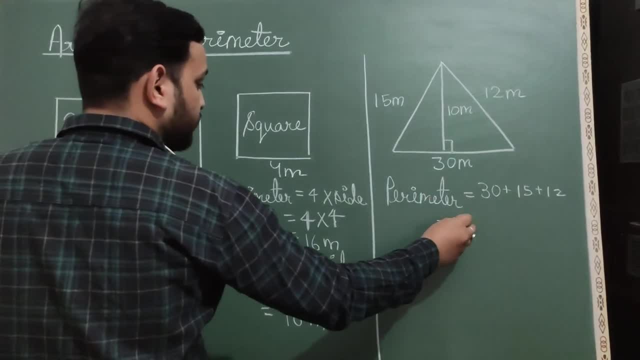 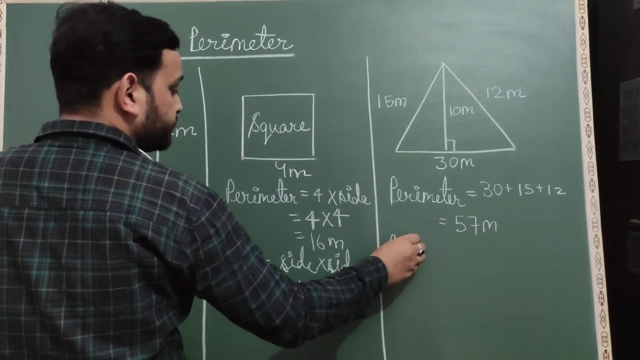 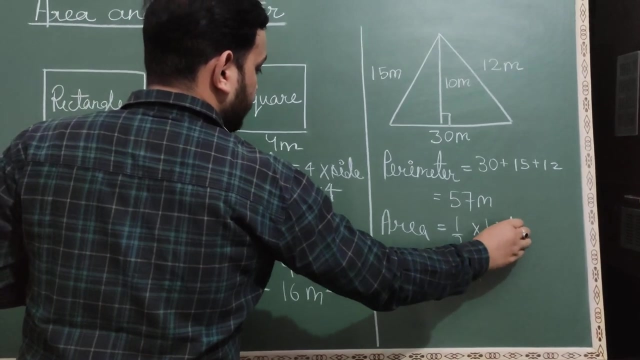 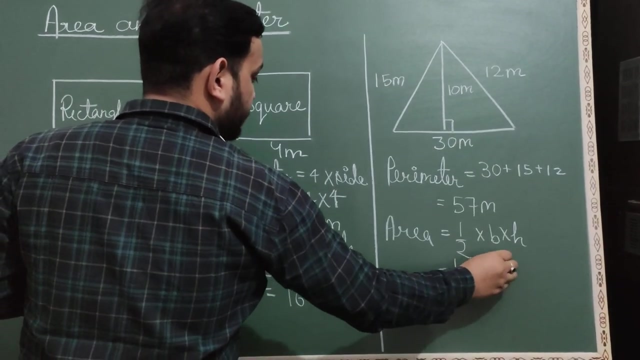 required to add all the sides. So 30 plus 15 plus 12, this will be 15.. 50, 7 meter. Now, formula of area of triangle. This is 1 upon 2. base into height. Now here, base is what is base here, This one is base, This is 30, and height. you can see what is. 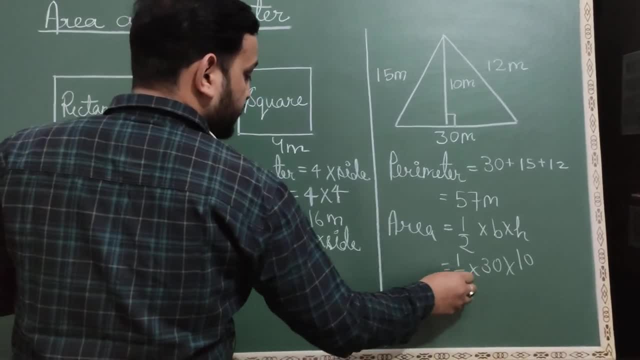 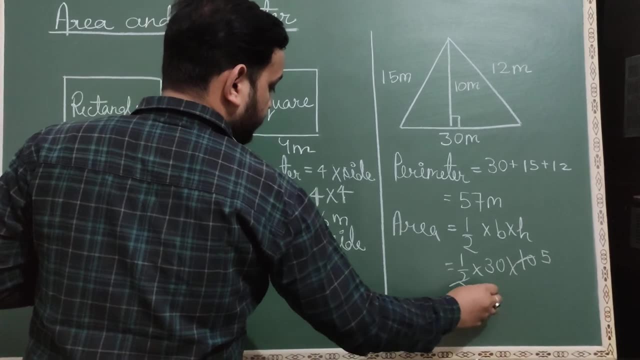 height, that is 10.. Now you can cut 2 5's are. that is 2 5's are 10.. So 3 5's are 10.. So 30 5's are 150 and it will be meter square. 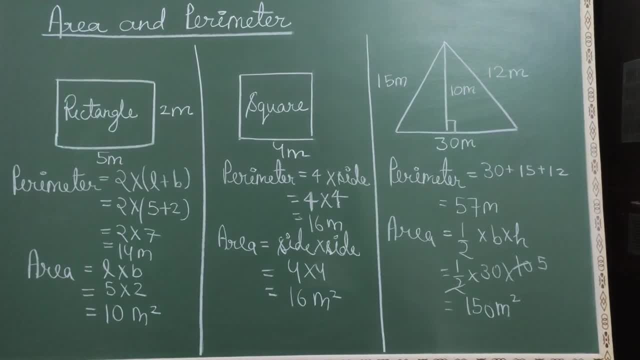 So in this way, you are required to find area and perimeter of the rectangle, square and triangle.